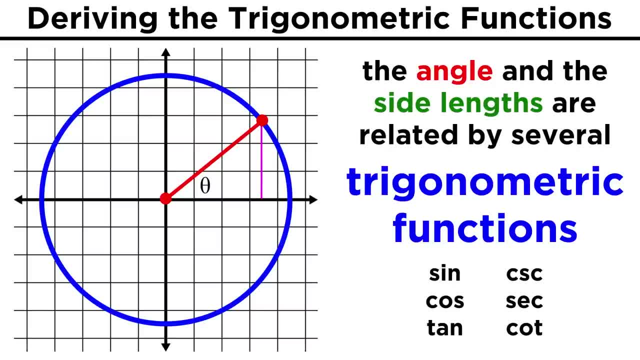 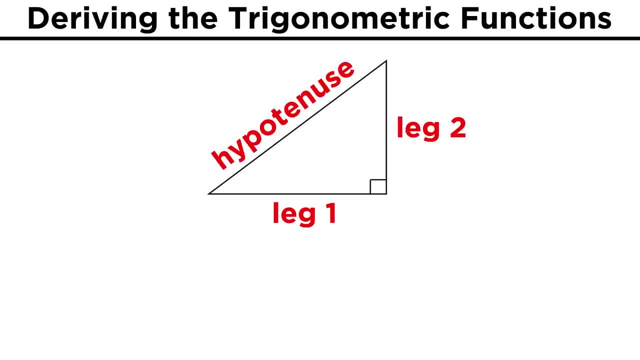 use trigonometric functions. Let's forget the circle. Let's draw a circle. Let's draw a circle for a second and just look at a right triangle. Here are the two legs: the hypotenuse and the angle of interest, theta. 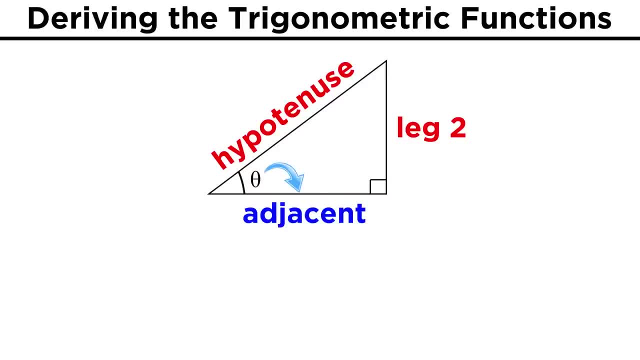 From now on, we will differentiate between the two legs by calling this one the adjacent leg, because it is the leg right next to the angle, and this one will be the opposite leg because it is directly opposite the angle. We will say that the sine of theta, which is abbreviated this way: S, I, N, is equal to: 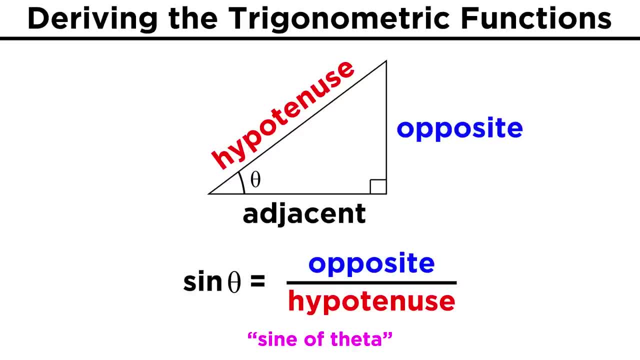 the sine of theta, which is abbreviated this way: S, I, N. Then the theta symbol will be equal to the length of the leg opposite the angle over the length of the hypotenuse. The cosine of theta will be equal to the length of the adjacent leg over the length of the. 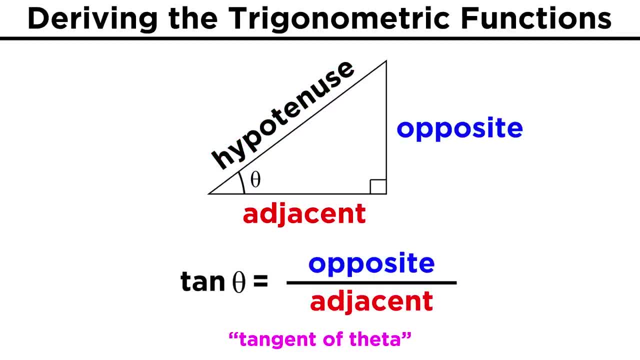 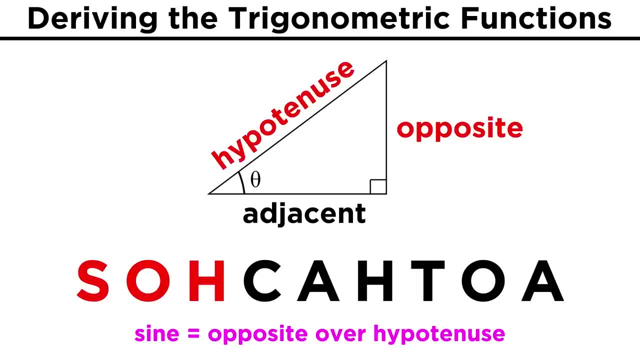 hypotenuse And the tangent of theta will be equal to the length of the opposite leg over the length of the adjacent leg. We can remember these definitions using the mnemonic SOHCAHTOA. These letters stand for sine opposite over hypotenuse, and then cosine adjacent over. 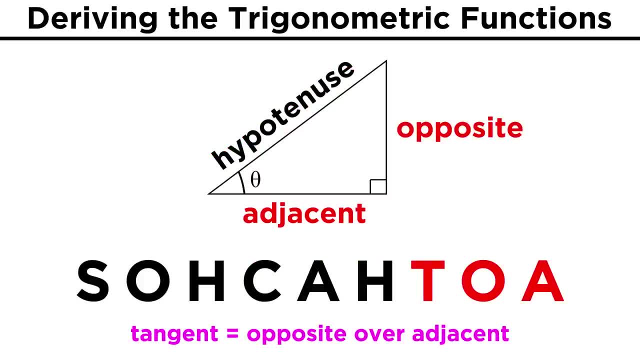 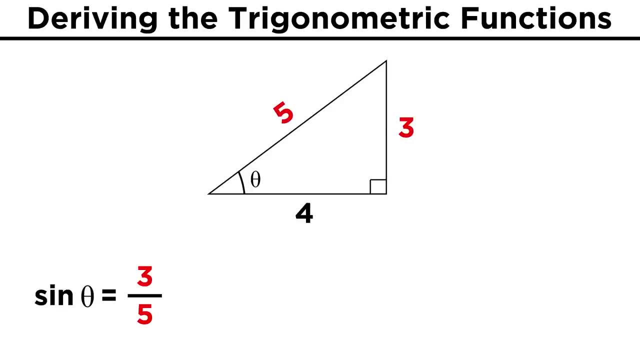 hypotenuse and, lastly, tangent. opposite over adjacent. Say it with me one more time, SOHCAHTOA. Looking at this triangle with sides of length three, four and five, sine of theta must be three over five. 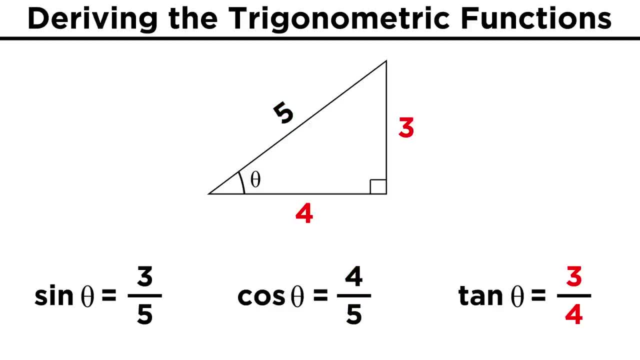 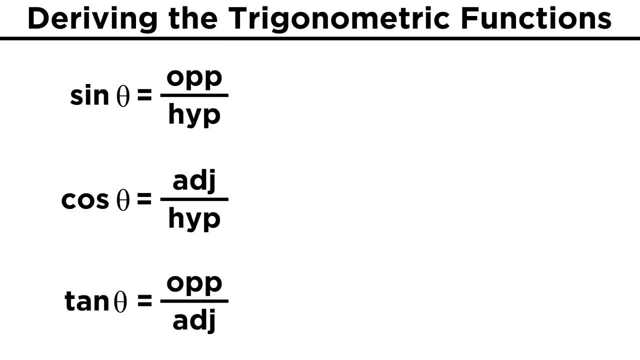 Cosine theta is four over five And tangent theta is three over four. Now we must learn the reciprocals of these functions. Cosecant is the reciprocal of sine. If sine is opposite over hypotenuse, cosecant is hypotenuse over opposite. 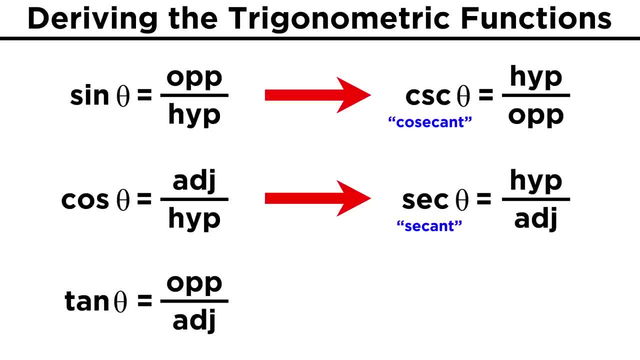 Secant is the reciprocal of cosine. so instead of adjacent over hypotenuse, it's hypotenuse over adjacent. Secant is the reciprocal of tangent. so instead of opposite over adjacent, it's adjacent over opposite. So we definitely have to memorize SOHCAHTOA, and then we just have to memorize which functions. 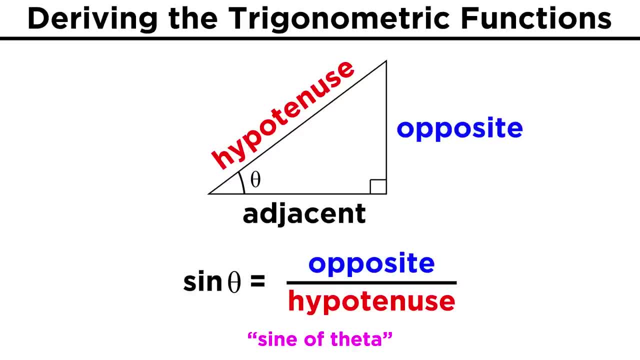 the sine of theta, which is abbreviated this way: S, I, N. Then the theta symbol will be equal to the length of the leg opposite the angle over the length of the hypotenuse. The cosine of theta will be equal to the length of the adjacent leg over the length of the. 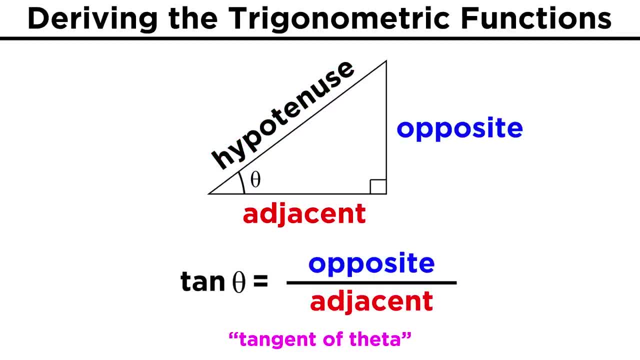 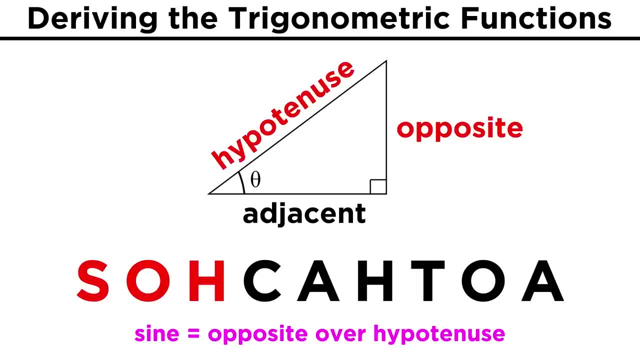 hypotenuse And the tangent of theta will be equal to the length of the opposite leg over the length of the adjacent leg. We can remember these definitions using the mnemonic SOHCAHTOA. These letters stand for sine opposite over hypotenuse, and then cosine adjacent over. 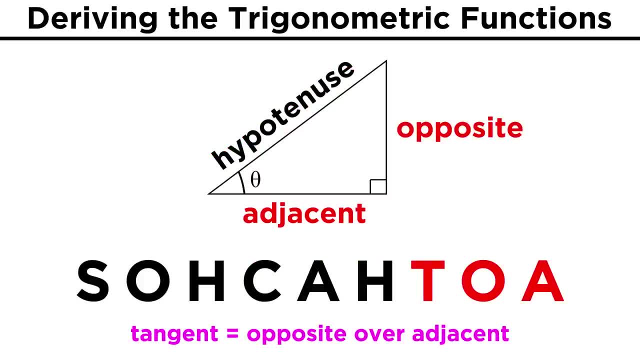 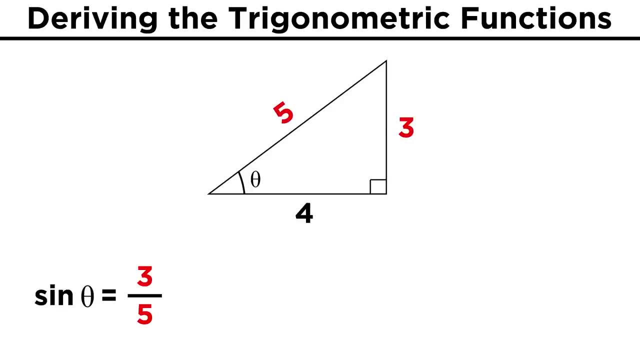 hypotenuse and, lastly, tangent. opposite over adjacent. Say it with me one more time, SOHCAHTOA. Looking at this triangle with sides of length three, four and five, sine of theta must be three over five. 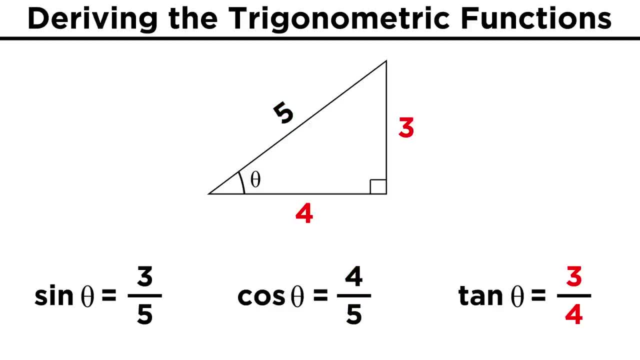 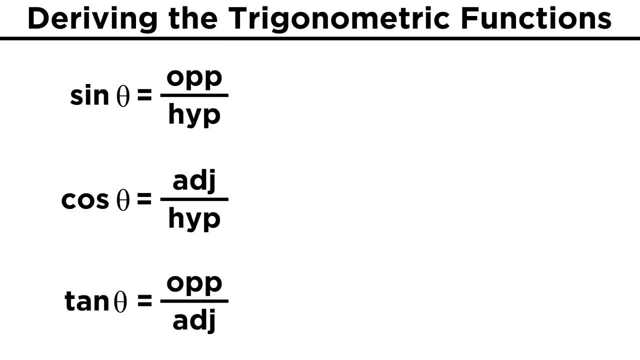 Cosine theta is four over five And tangent theta is three over four. Now we must learn the reciprocals of these functions. Cosecant is the reciprocal of sine. If sine is opposite over hypotenuse, cosecant is hypotenuse over opposite. 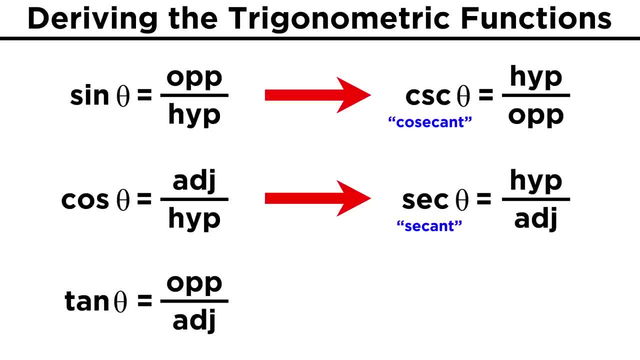 Secant is the reciprocal of cosine. so instead of adjacent over hypotenuse, it's hypotenuse over adjacent. Secant is the reciprocal of tangent. so instead of opposite over adjacent, it's adjacent over opposite. So we definitely have to memorize SOHCAHTOA, and then we just have to memorize which functions. 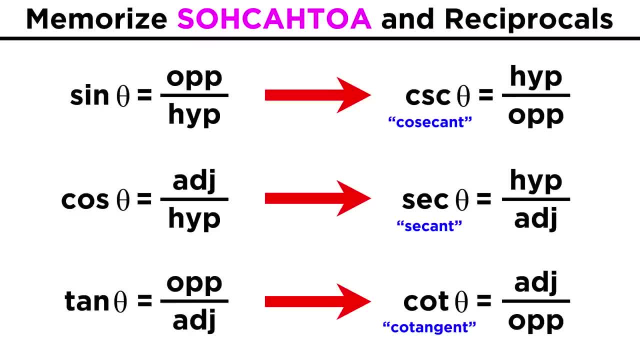 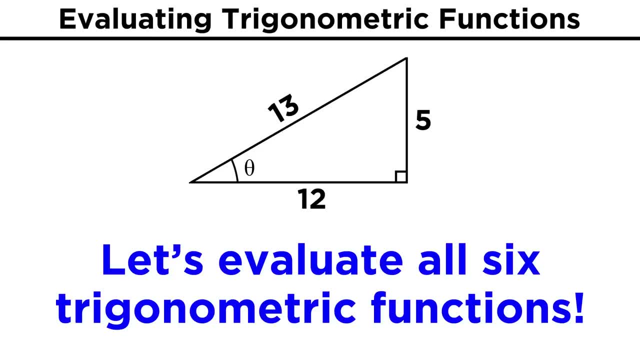 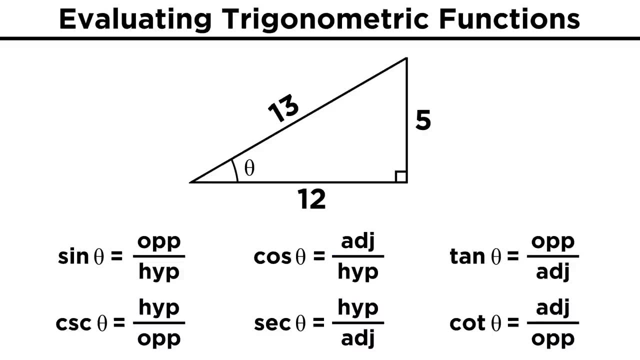 are the reciprocals of these three, since we can just flip these ones to get the others. So let's take this triangle with sides of five, twelve and thirteen and evaluate all six trigonometric functions. We can place all the letters first to represent the sides involved in each calculation. 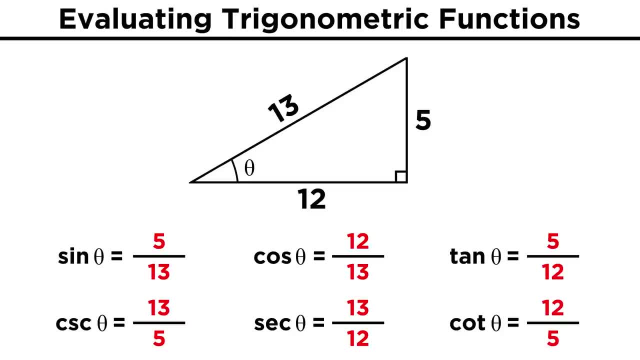 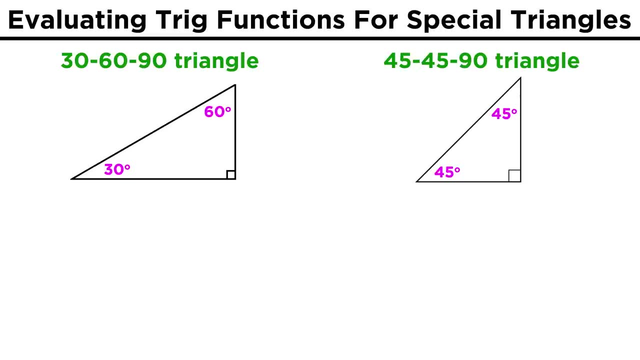 Then we fill in the respective numbers, See that there isn't really any reducing to be done. so these are the six values we end up with. So now that we know how to evaluate these functions, let's look at two special triangles that will come up a lot. 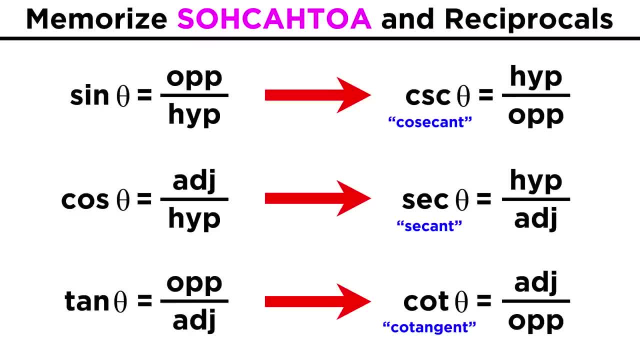 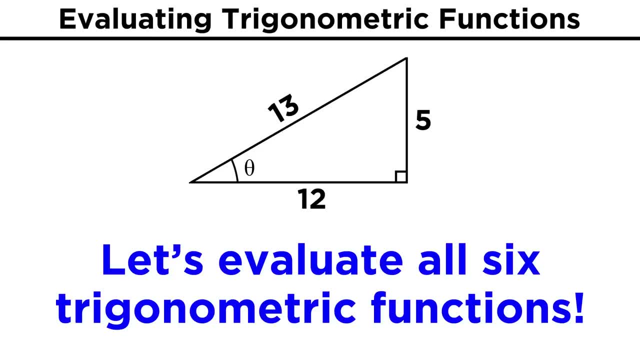 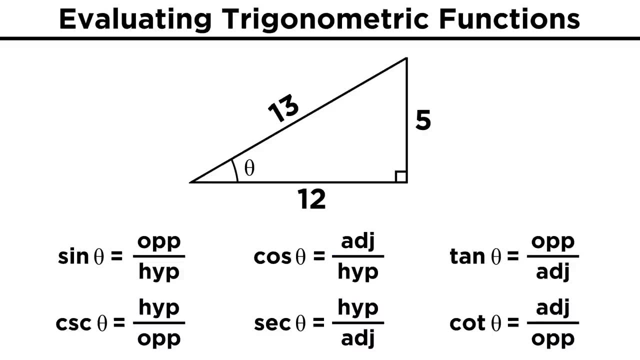 are the reciprocals of these three, since we can just flip these ones to get the others. So let's take this triangle with sides of five, twelve and thirteen and evaluate all six trigonometric functions. We can place all the letters first to represent the sides involved in each calculation. 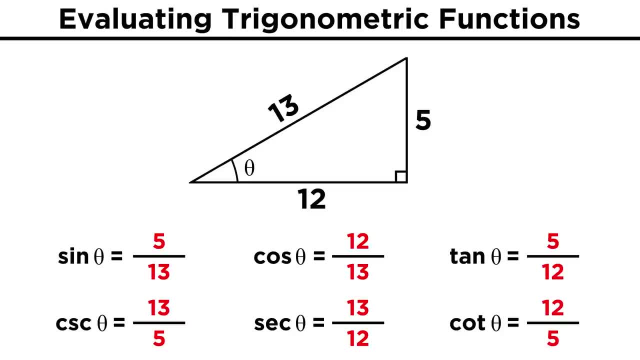 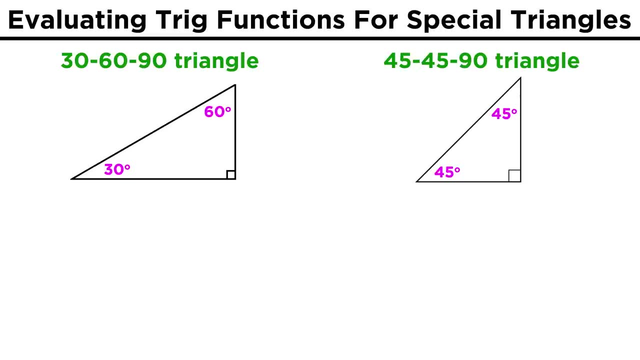 Then we fill in the respective numbers, See that there isn't really any reducing to be done. so these are the six values we end up with. So now that we know how to evaluate these functions, let's look at two special triangles that will come up a lot. 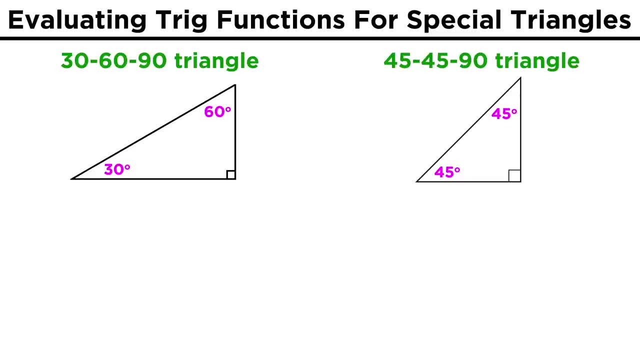 These are the thirty-sixty-ninety-six. Let's look at them one by one. The forty-five-forty-five-ninety triangle and the forty-five-forty-five-ninety triangle. Let's find the sine cosine and tangent for these three angles. 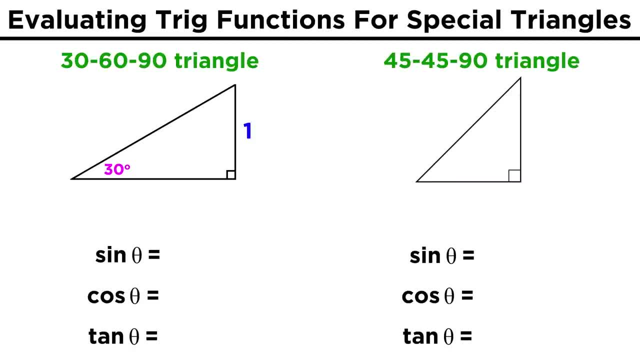 First, for thirty degrees, As we recall from geometry, if the shorter leg of this triangle has a length of one, the other sides must be root three and two. Therefore, the sine of thirty is one half. the cosine of thirty is root three over two. 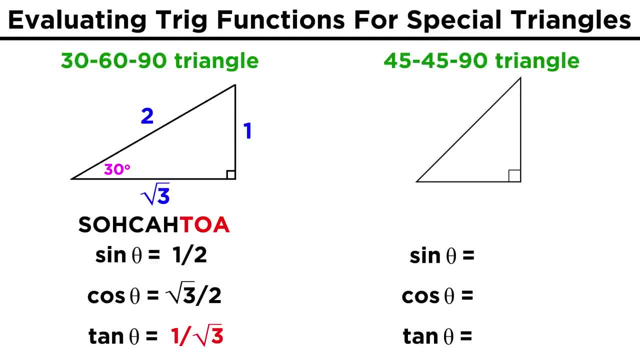 and the tangent of thirty is one half. The tangent of thirty is one over root three, but since we don't like roots in the denominators, we multiply by root three over root three, which gives us root three over three. We can use the same triangle to evaluate the same functions for the sixty degree angle. 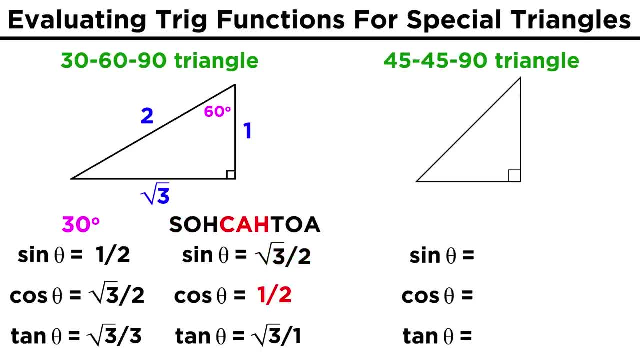 Sine of sixty is root three over two, cosine of sixty is one half and tangent of sixty is root three over one, or simply root three. Now let's do the same for the forty-five degree angle in this other special triangle. As we recall, if one leg of this triangle is equal to one, the other sides must be one. 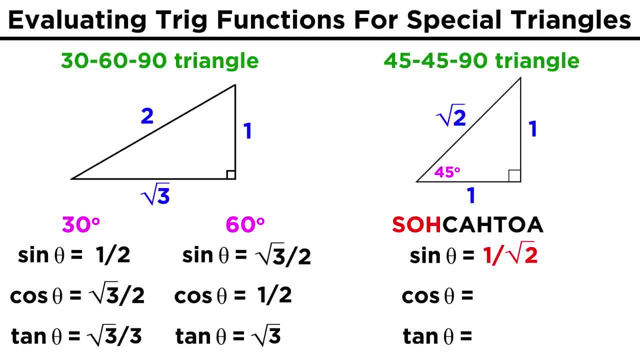 and root two. So the sine of forty-five is one over root two. but we multiply by root two over root two to get root two over two, and the cosine of forty-five will give us the same value, since the two legs have the same length. 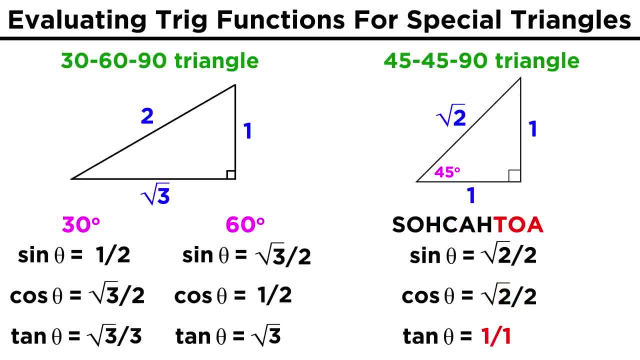 The tangent of forty-five is one half and the tangent of forty-five is one half and the tangent of forty-five is one half. tangent of forty-five will be one over one or simply one. These triangles will come up again and again. so these values of sine and cosine will be. 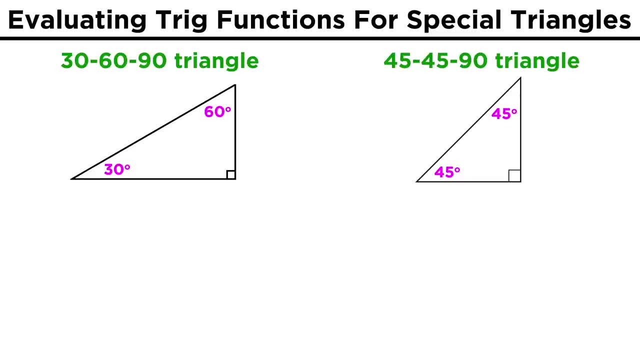 These are the thirty-sixty-ninety-six. Let's look at them one by one. The forty-five-forty-five-ninety triangle and the forty-five-forty-five-ninety triangle. Let's find the sine cosine and tangent for these three angles. 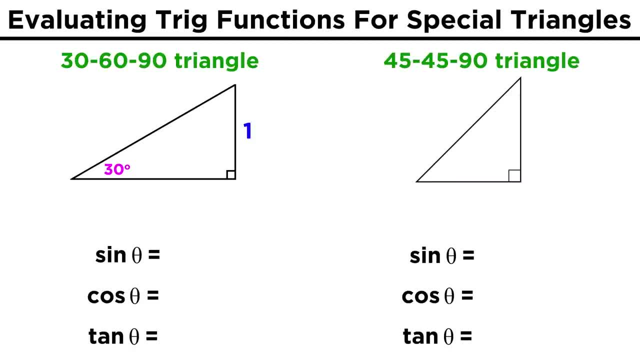 First, for thirty degrees, As we recall from geometry, if the shorter leg of this triangle has a length of one, the other sides must be root three and two. Therefore, the sine of thirty is one half. the cosine of thirty is root three over two. 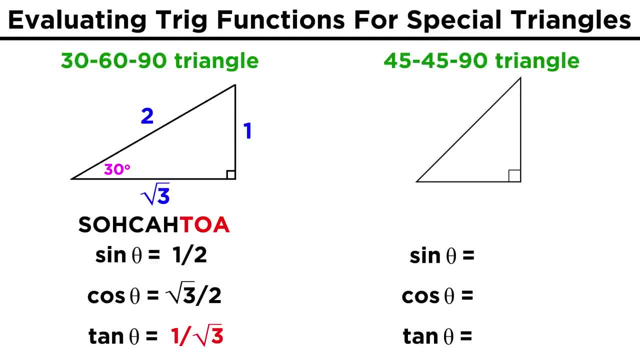 and the tangent of thirty is one half. The tangent of thirty is one over root three, but since we don't like roots in the denominators, we multiply by root three over root three, which gives us root three over three. We can use the same triangle to evaluate the same functions for the sixty degree angle. 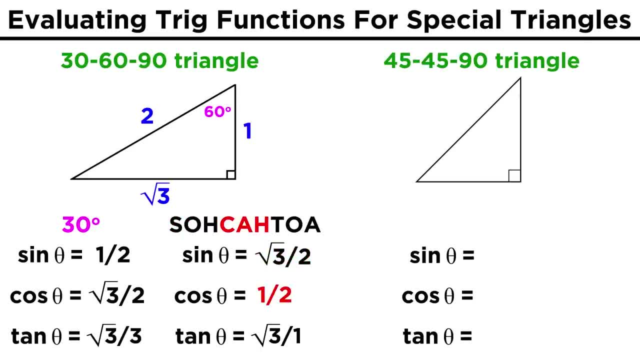 Sine of sixty is root three over two, cosine of sixty is one half and tangent of sixty is root three over one, or simply root three. Now let's do the same for the forty-five degree angle in this other special triangle. As we recall, if one leg of this triangle is equal to one, the other sides must be one. 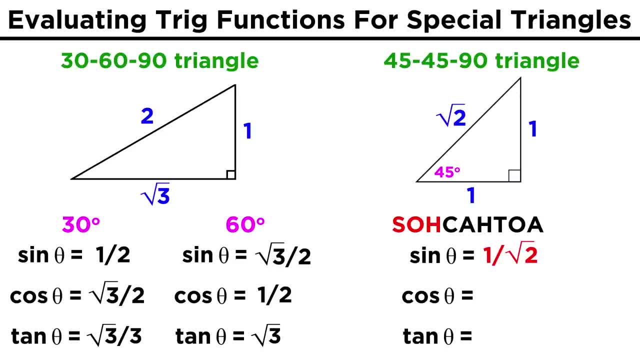 and root two. So the sine of forty-five is one over root two. but we multiply by root two over root two to get root two over two, and the cosine of forty-five will give us the same value, since the two legs have the same length. 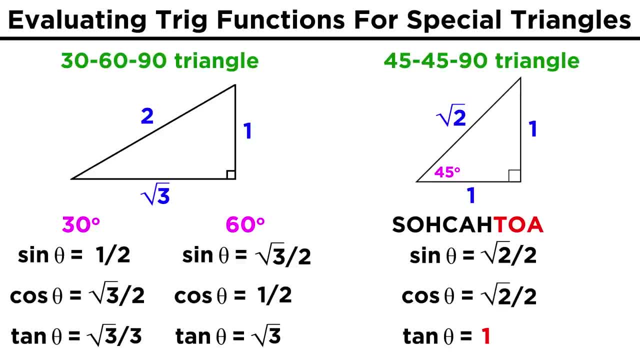 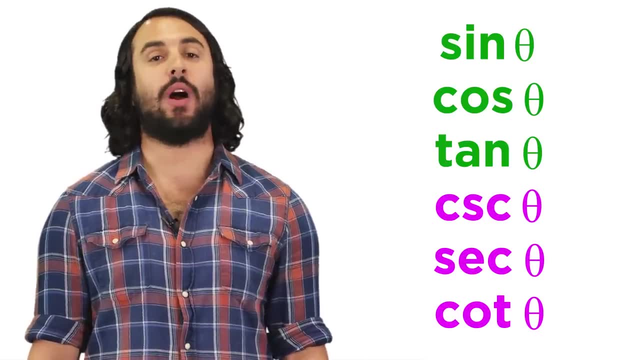 tangent of forty-five will be one over one or simply one. These triangles will come up again and again, so these values of sine and cosine will be very common as well. Ideally, we now understand what these six trigonometric functions are and how to calculate.